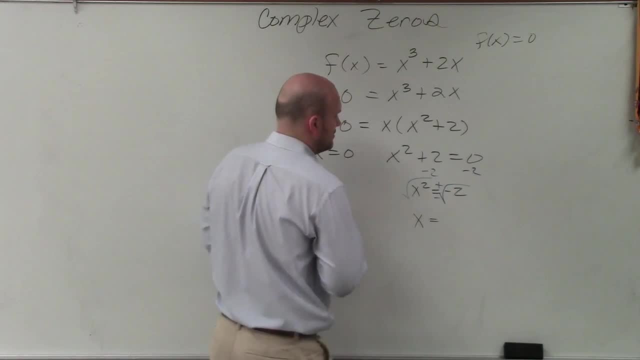 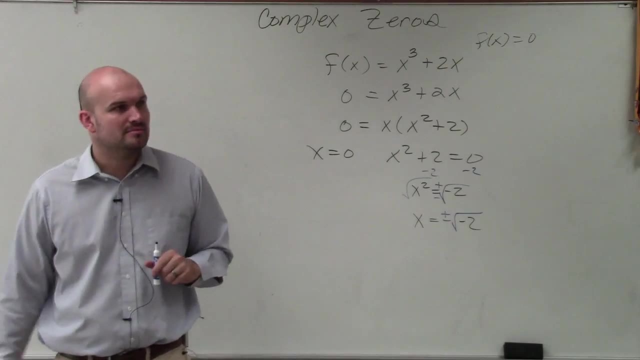 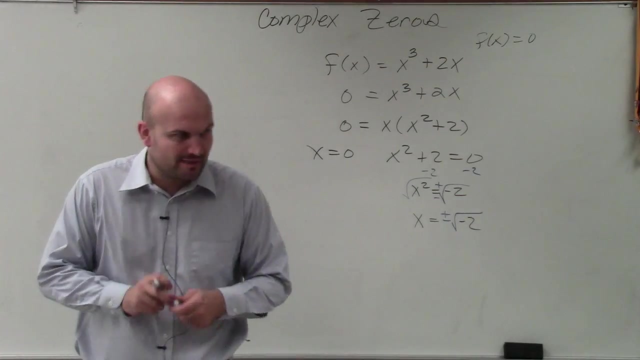 Yes, Can we have Jake Switzer to the main office for a few minutes, And he will be returning, OK. OK, So we have plus or minus the square root of negative 2.. However, ladies and gentlemen, if you remember from back in your days of algebra 2,, 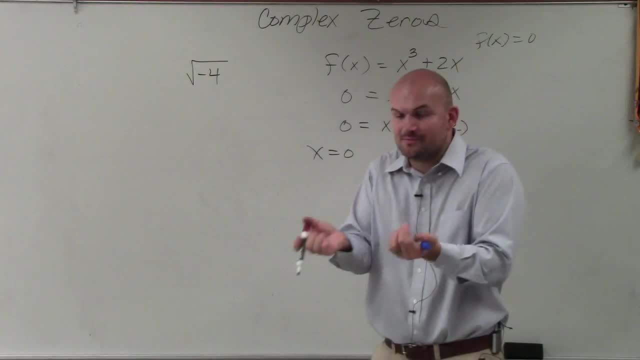 let's just look at negative 4.. There's not two numbers that are exactly the same. There's not any number that's exactly the same that multiplies to give you negative 4.. You can think of 2 times 2 as positive 2.. 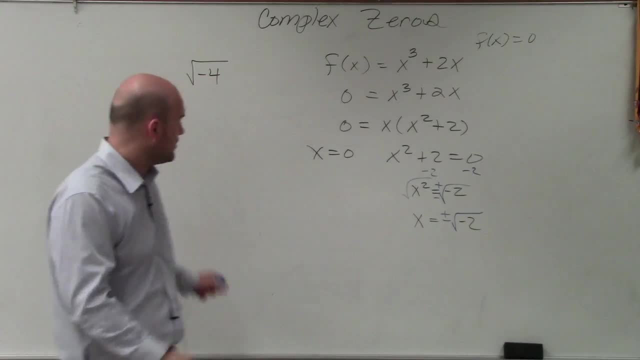 Negative 2 times negative 2 is positive 4.. So the only way to get negative 4 would have to be negative 2 times 2, but those numbers are not exactly the same. So what we do when we're simplifying something, 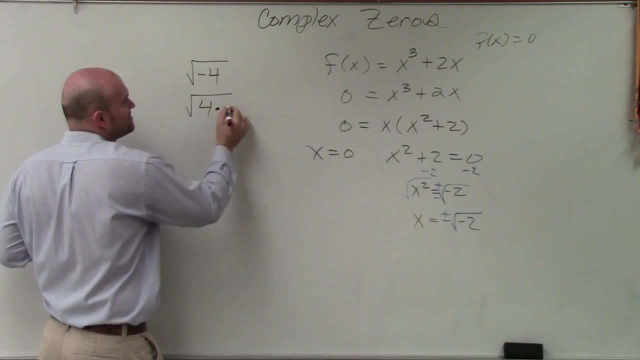 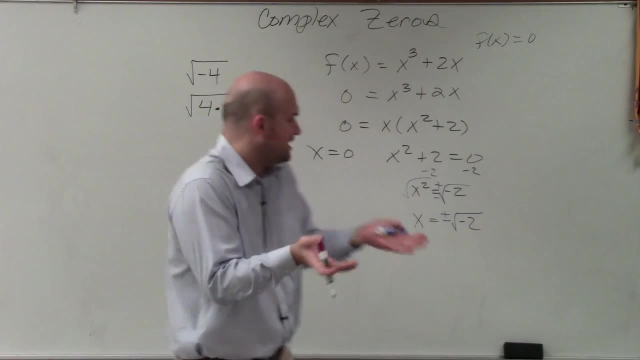 like this is: we rewrite this as 4 times negative 1, where negative 1 represents our imaginary units, because you cannot take the square root of a negative 1.. So whenever you have the square root of a negative number, rewrite it. 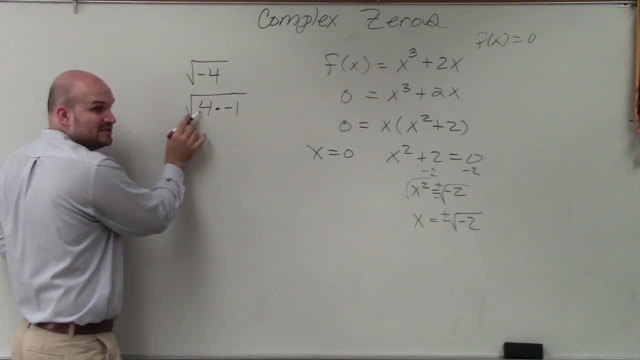 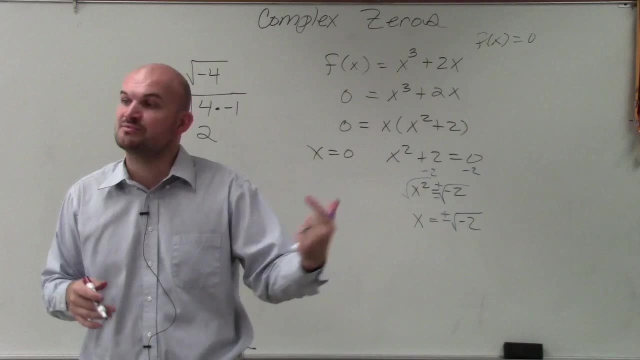 Write it as the positive times negative 1.. Because now can you take the square root of 4?? Yes, You cannot take the square root of negative 1 in the real number system, so we create an imaginary number or imaginary unit i. 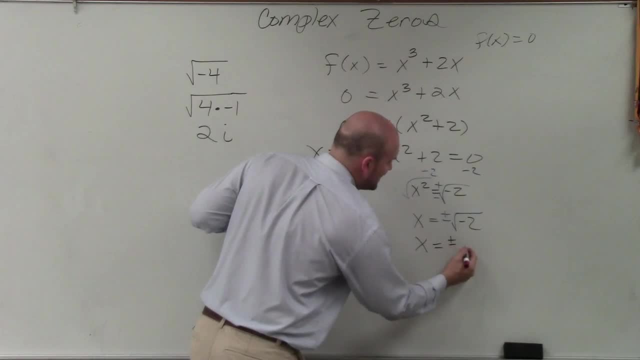 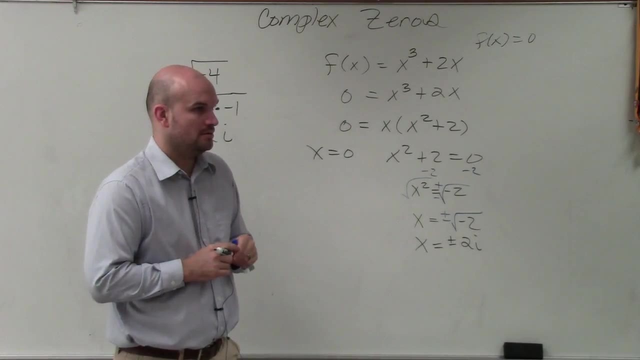 So in this case I have x equals plus or minus 2i Question: What would be pi times 2?? 2 is a square number. Oh no, I'm sorry, It's square root 2, right, Sorry? 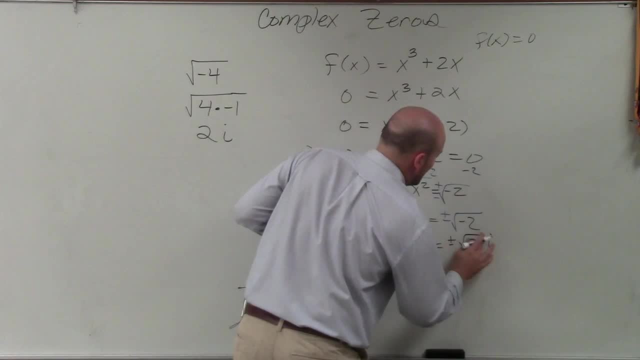 Thank you. Square root of 2i. And a lot of times we write the i in front of the square root because the main important thing is what students will do is they'll write it like that and they'll accidentally put the square root above. 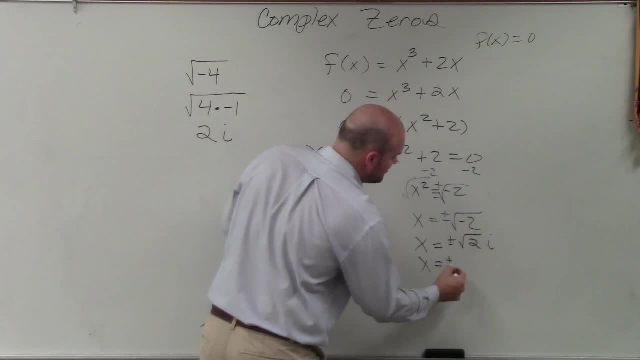 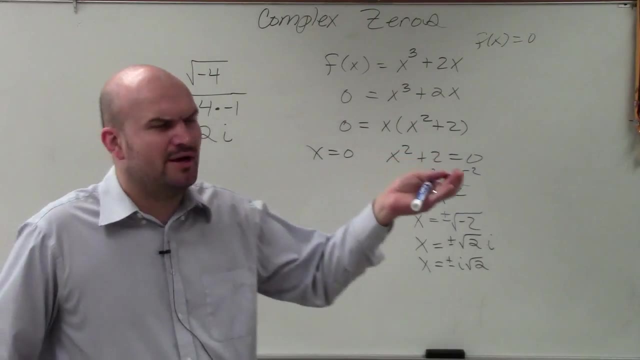 So a lot of times when you have the square root, we'll write it as plus or minus i- square root of 2.. When you're usually dealing with other numbers, we don't write x3.. We write 3x, Right. 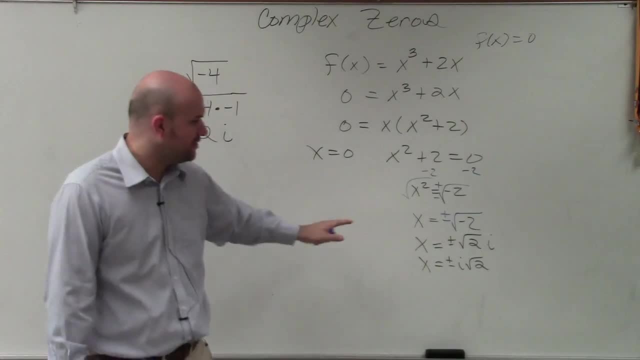 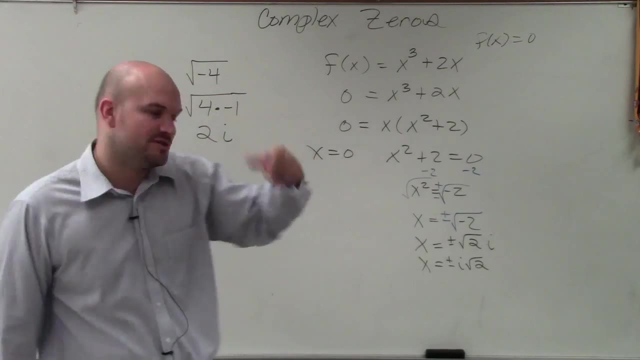 So we usually like to write the i in front. However, with square roots, students will make the mistake and always put the i, so we like to write the i in front. Now, let's go and think about this, though. to our problem.